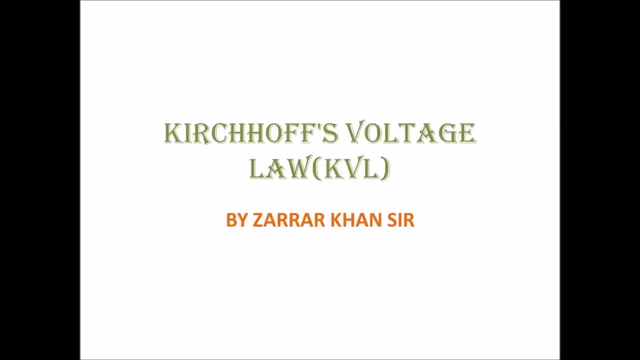 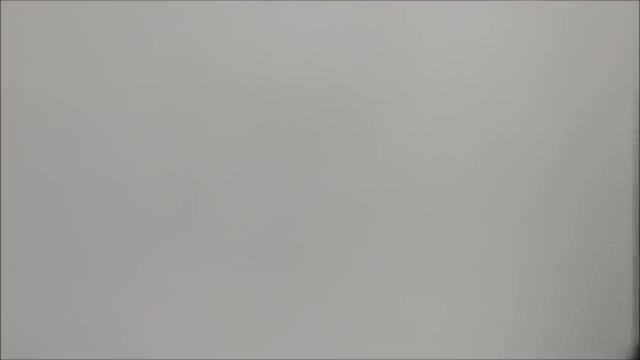 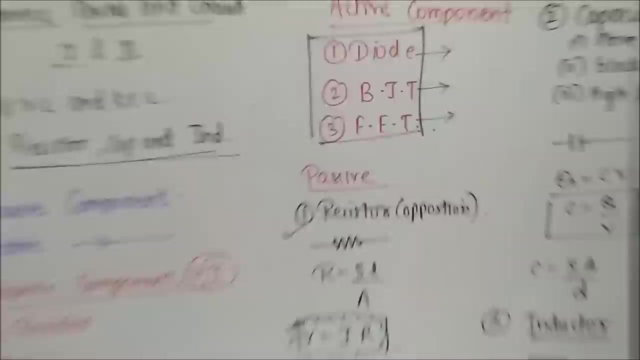 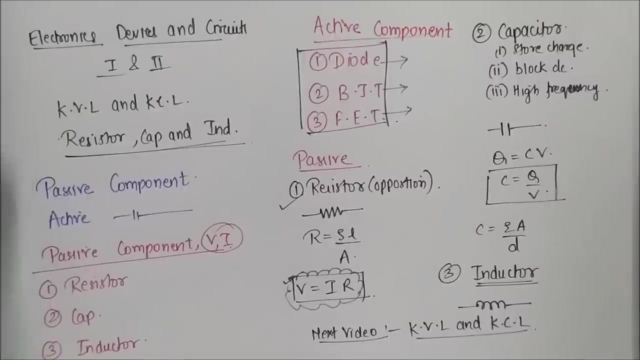 Hello, as I said, we will be discussing KVL and KCL in the next lecture. Today we will be discussing KVL and KCL just to revise what we have already seen: Electronics devices and circuit. We will be trying to study electronics devices and circuit And we will be studying. 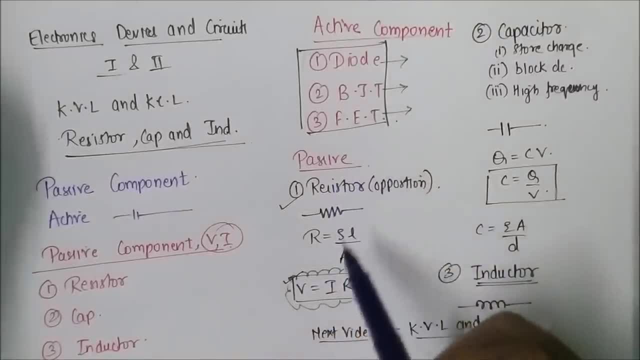 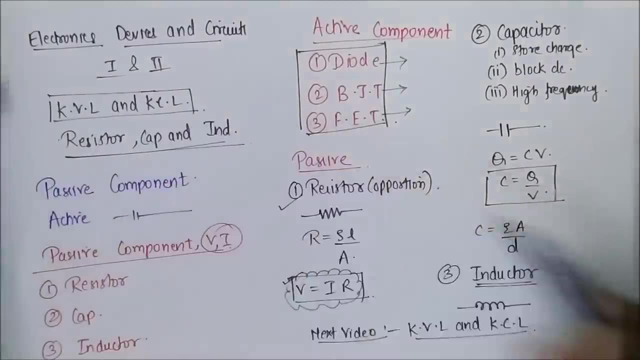 BJT and FET in detail, But for that we will be requiring basic, fundamental related to V, equal to IR and some important components such as or not component, it is equation- or to understand how to apply KVL and KCL in different circuits. Okay, so let's start with. 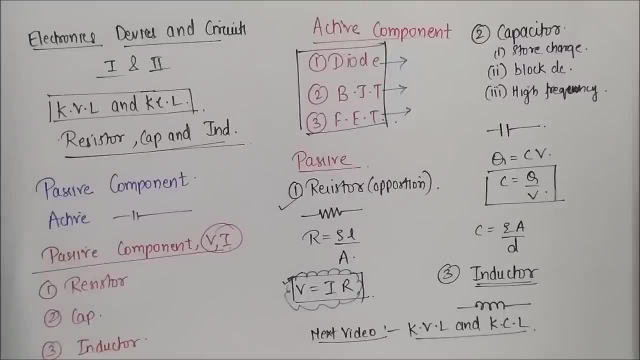 KVL and KCL, But I will be teaching only KVL in this circuit. If you understand and if you want to apply KVL or if you need KCL, then please do message me or write down in comment. In sha Allah, I will upload KCL or shortcut for. 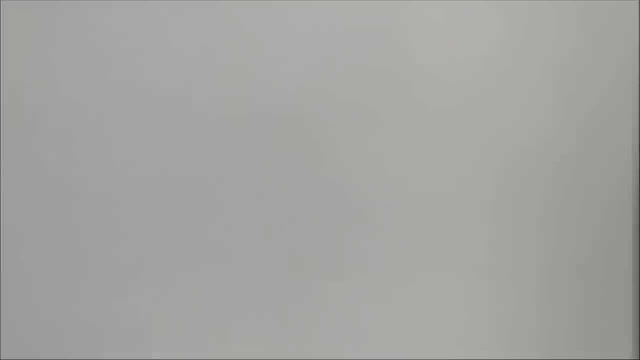 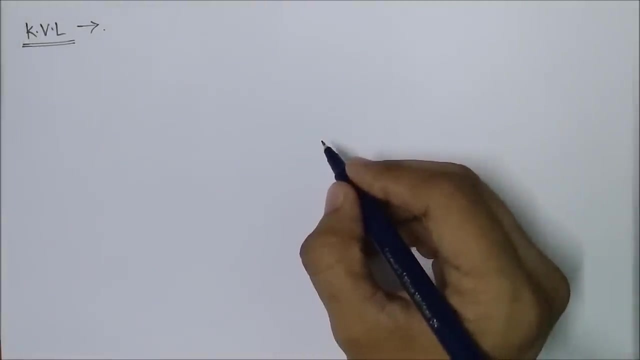 KCL also. Okay, so I will be teaching you KVL right now, Guys, what do you mean by KVL? So, guys, what do you mean by KVL? See, student know basically the full form of KVL. it is Kirchhoff voltage law. But being an engineer, 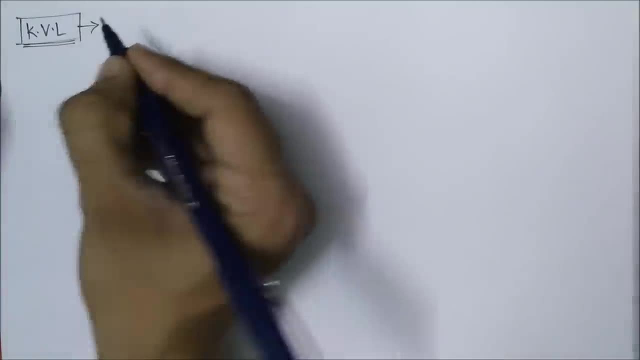 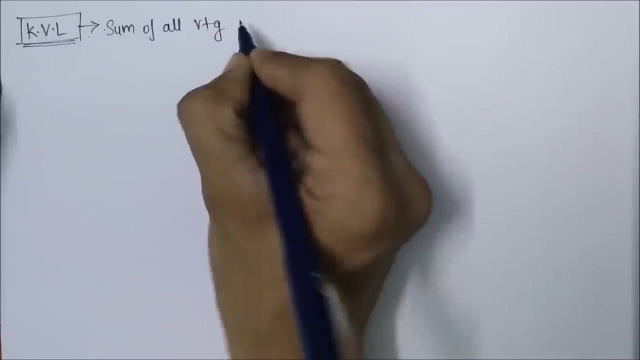 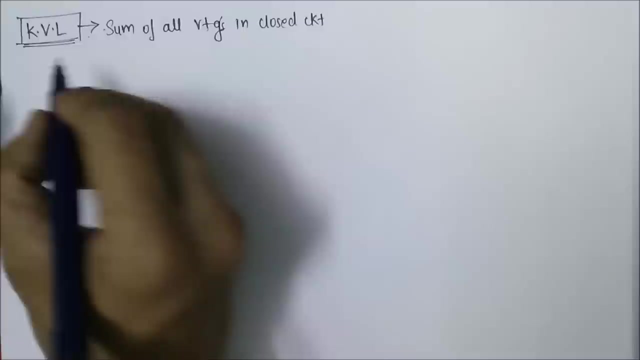 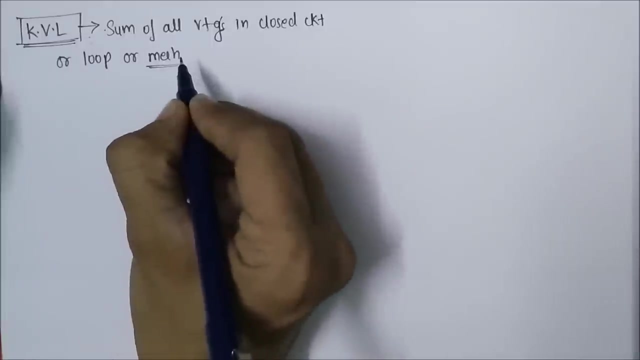 Okay, We need to understand what law says. It says the algebraic sum of all the voltages, which mean sum of all voltages in closed circuit, or loop or mesh, and we all know mesh is the smallest loop which cannot be further divided. So sum of all voltages in a closed circuit. 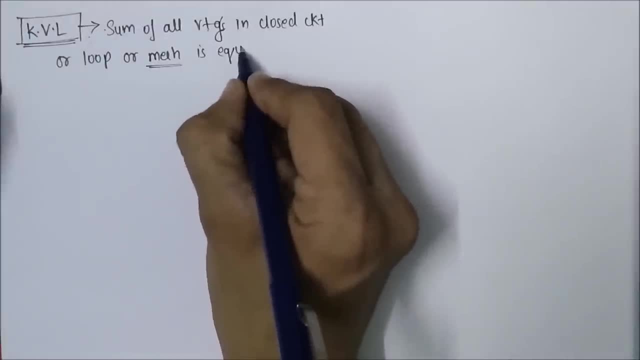 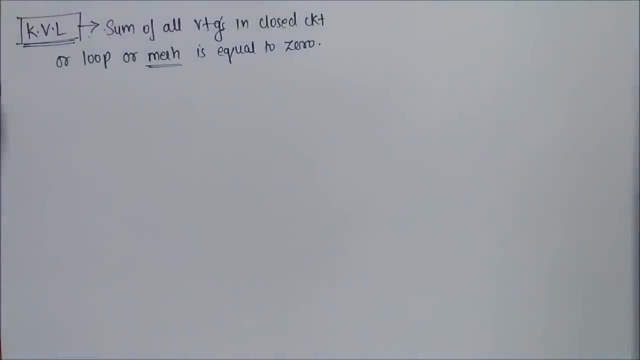 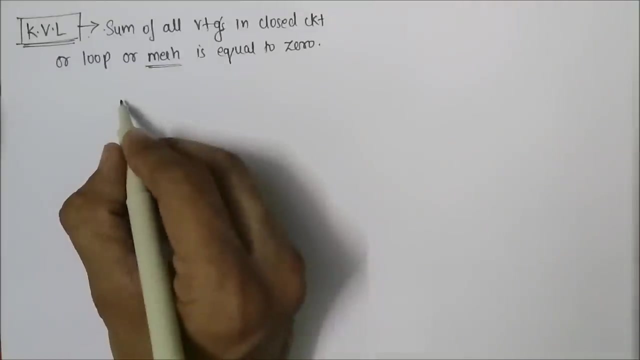 or loop or mesh. So let's suppose I tell you that KVL is equal to 0.. Okay, This is the definition. what does law means? Now I will be giving you an example and shortcut to remember how to apply KVL. Okay, let's assume this is the circuit in. 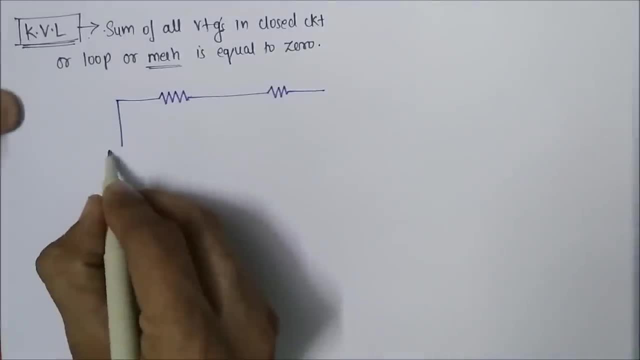 which we need to apply. See, guys, there are two types of sources. they something called dependent and independent source. So, with I'll be teaching you, As I said, I will be teaching you the circuit and the independent source. So let's run. 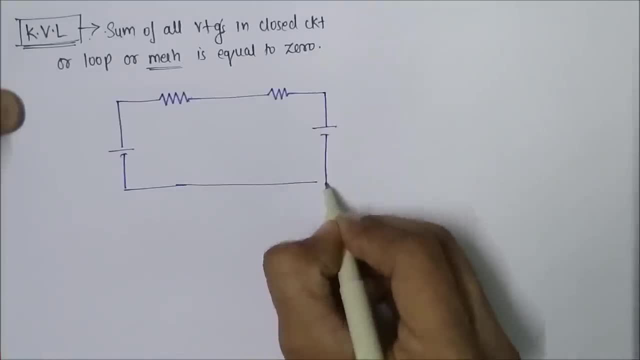 around. So this is the circuit in which we need to apply. for See, guys, there are two types of sources and something that is dependent and independent source. So I will be teaching you, As I said, be teaching a fundamental related what is required in EDC, so I'll be teaching. 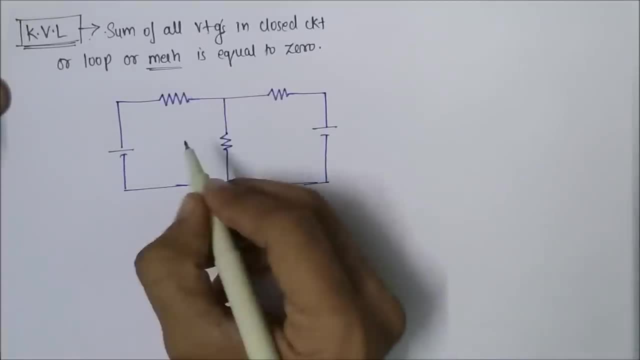 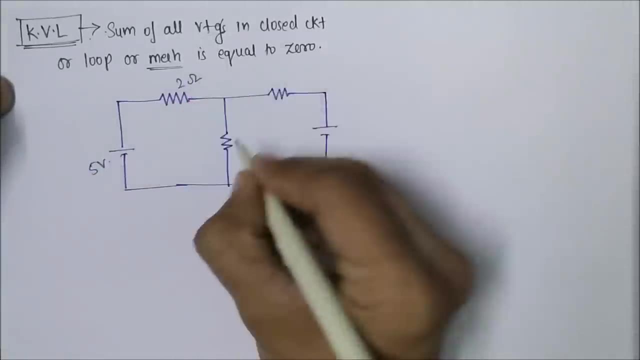 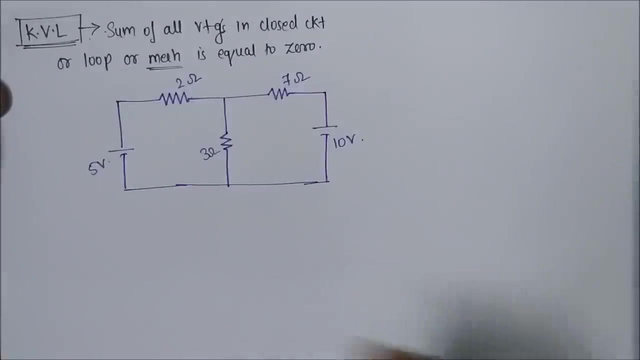 you only independent source. I won't be rest, I won't be teaching you dependent, so so assume this is voltage to be a 5 volt, 2 ohm, 3 ohm, 7 ohm and 10 volts. so this are, this is the in this, this circuit you need to find current using. 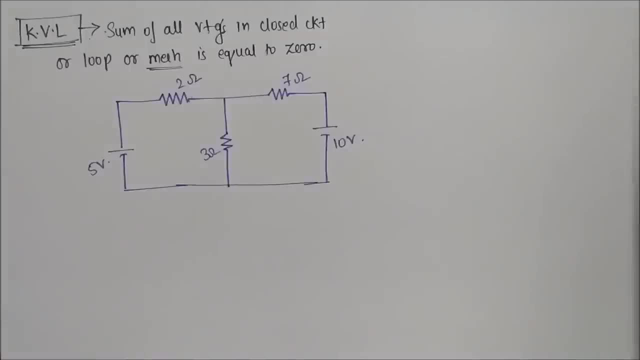 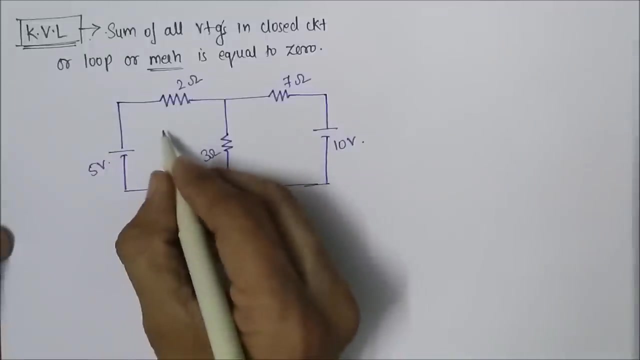 Kirchoff voltage law. so let's apply Kirchoff. one day, love, I'll be giving you a shortcut after completion of this, this circuit, but we still start first with the basic, what we have already studied. so, guys, assume any direction in which current is flowing. suppose current is flowing in the direction. assume let's. 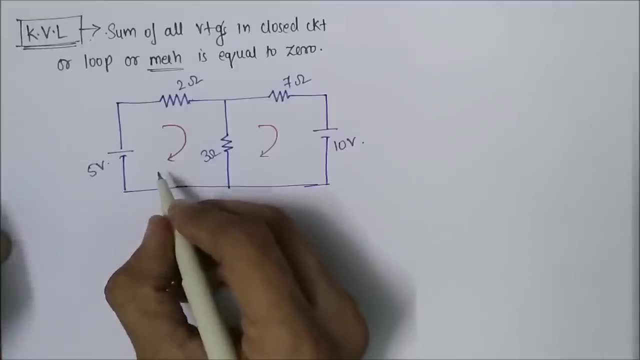 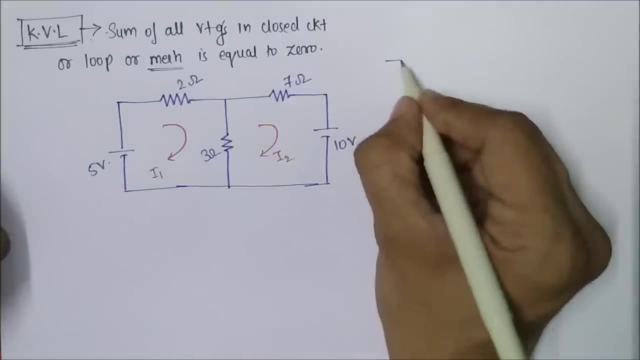 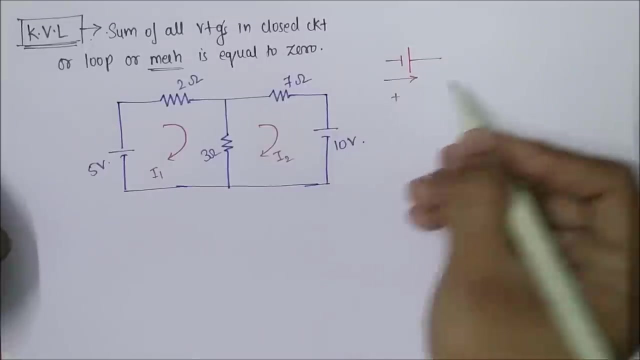 say I will take it clockwise and then we'll take and the clockwise. if you want, you can take any clockwise. so I'll assume this current to be I1 and assume this current to be. I do do remember if current flows from lower potential to higher potential will assume to be positive and if it moves. 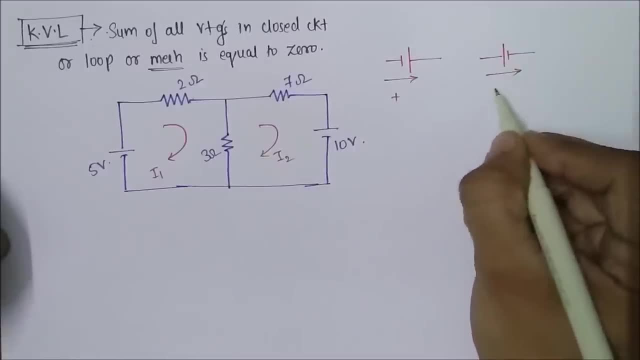 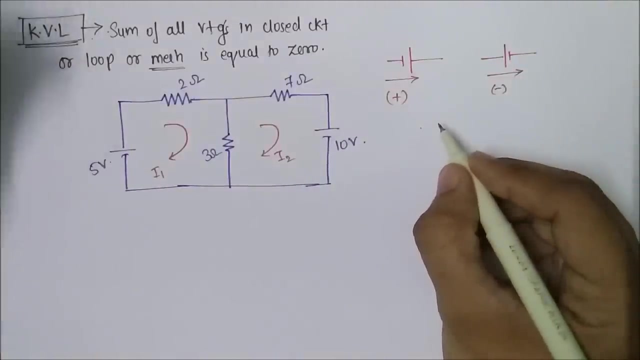 from positive or higher potential to lower potential, will assume to it to be negative. just remember this true thing and further work will be a. further efforts will be reduced, okay, and every time if you see a resistance, assume it to be a voltage drop, since the resistance opposes the flow of current. 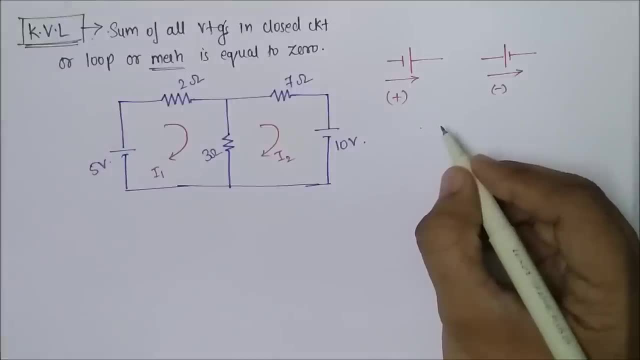 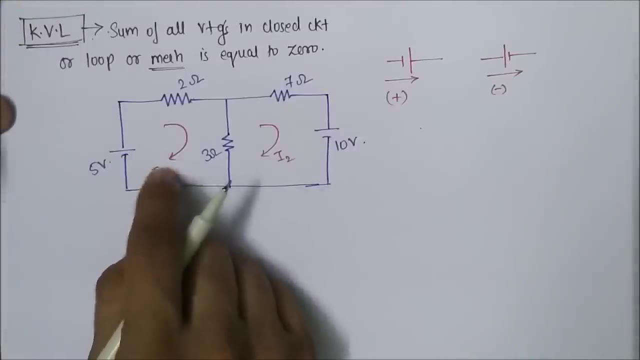 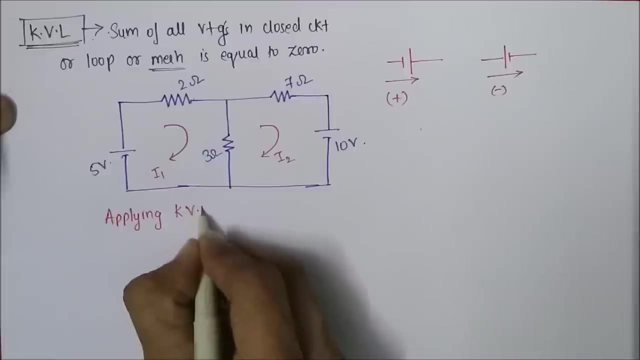 assume every time, whenever you see resistance, assume it to be have a have. assume it to be have a voltage drop. so, guys, let's start. so I am starting from here. I will be in first loop, so I'll write applying KVL in loop 1. okay, 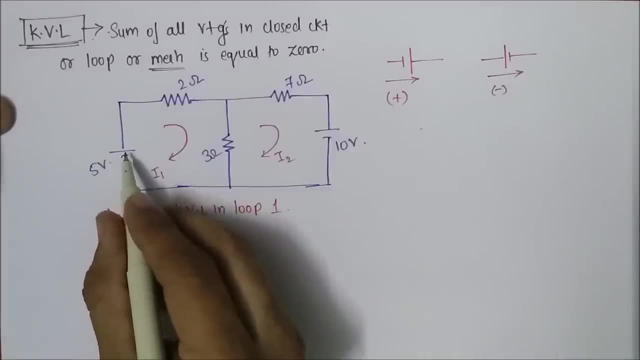 applying KVL in loop 1. so if I move from negative to positive, you will see that I have a voltage drop, so I will write: applying KVL in loop 1. okay, applying KVL in loop 1. so if I move from negative to positive. 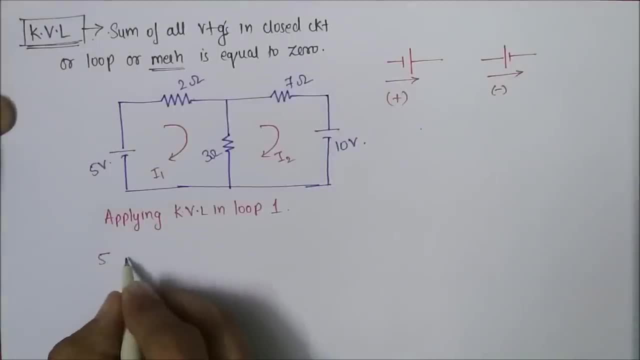 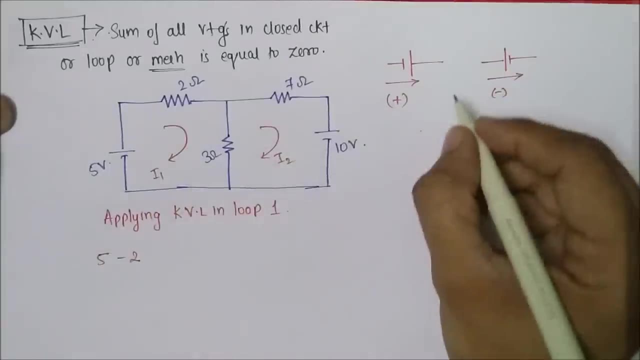 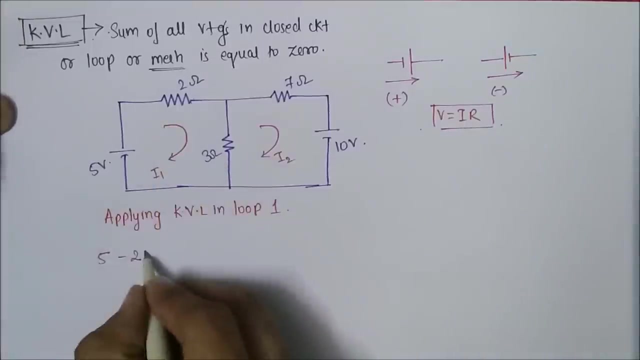 I'll take it out to be positive. so I'll take 5, and every time you see a resistance you should write minus 2, since V equal to. I do remember this equation, it is very important: V equal to IR. so minus 2 times I 1, minus 3 times. 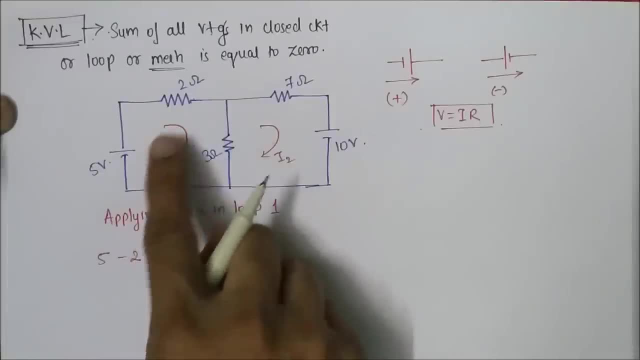 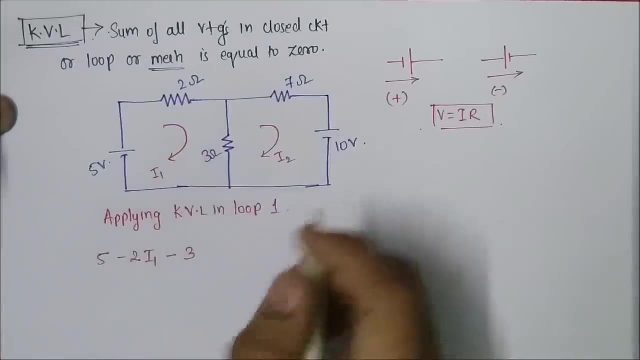 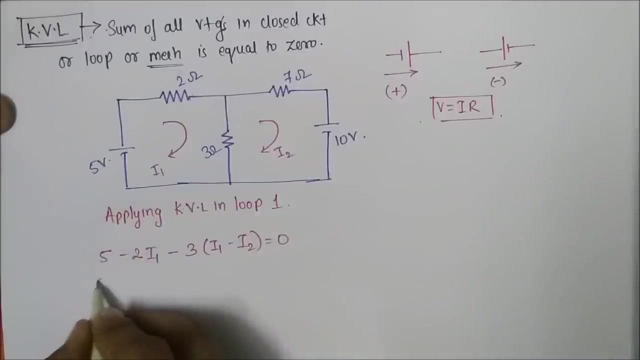 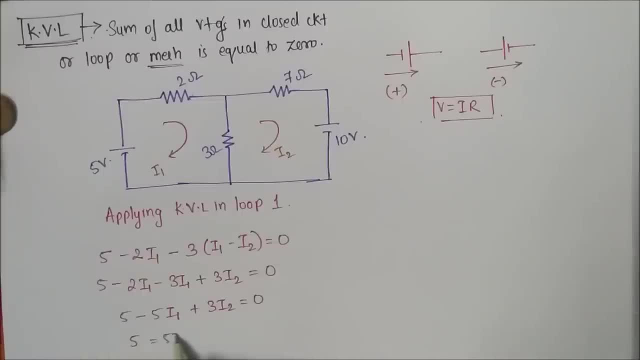 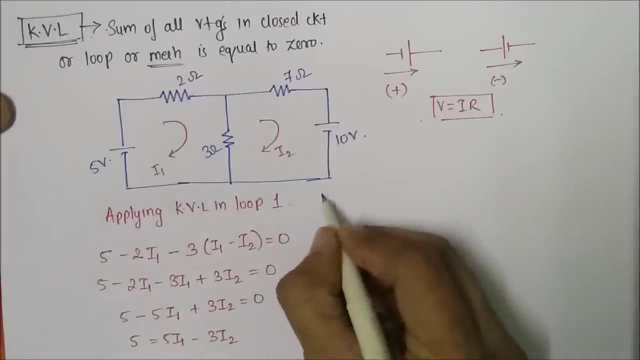 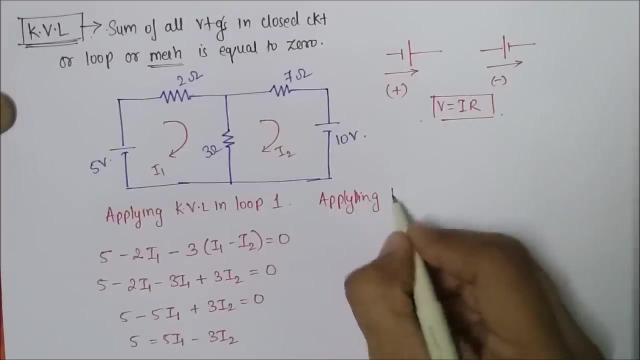 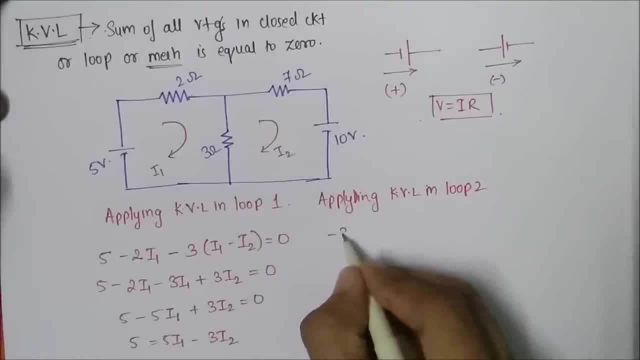 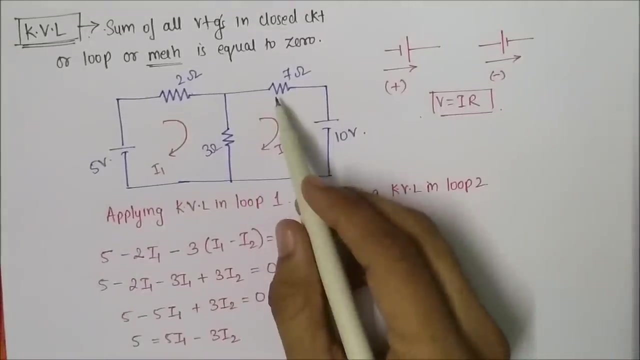 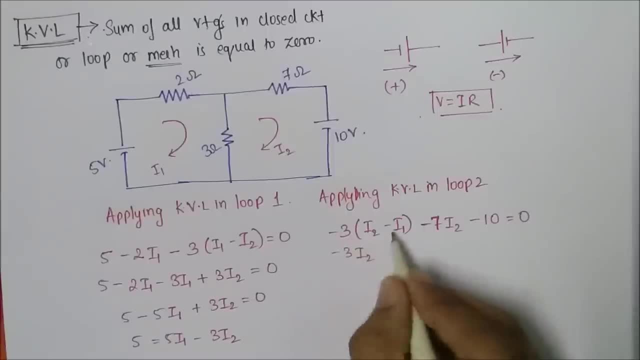 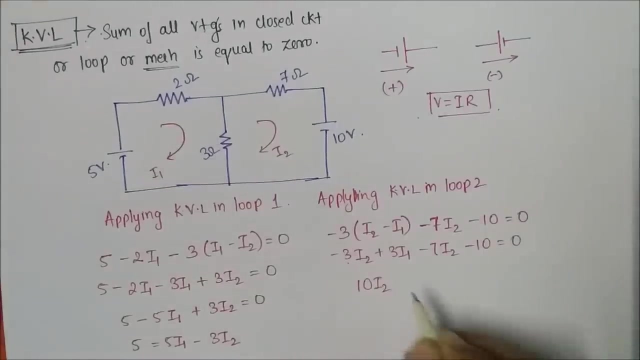 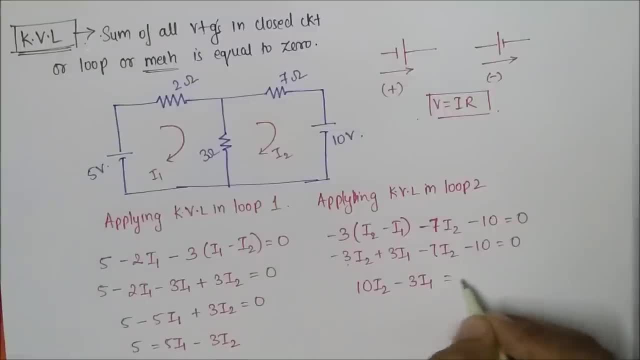 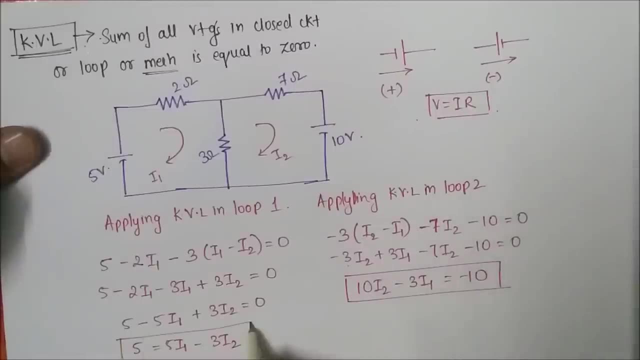 plus 10, I 2 minus 3, I 1 equal to minus 10. so this is another equation. so this is equation number 1, this is equation number 2, and we know how to solve simultaneously simultaneous equation in calculator. but I now please, please, make. 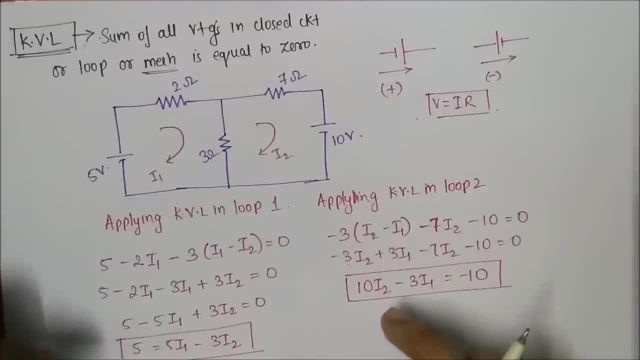 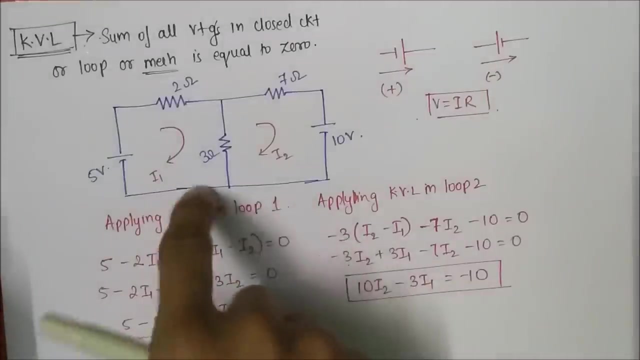 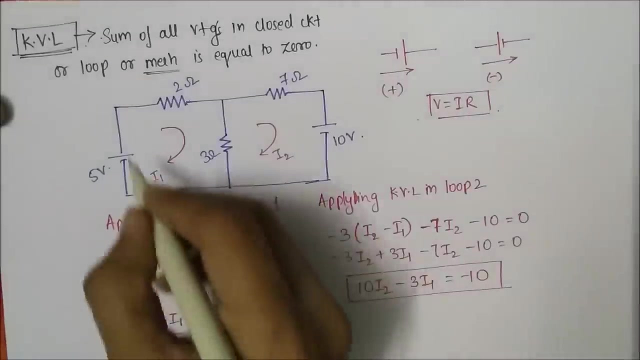 sure how to write this equation in fast manner. this is important for GE or GE student also and for NE student also. you can, how you can directly write down the final equation of this two loop and for also BW first year graduates. so it's very simple, guys. do remember if I am in first loop, count the total number of. 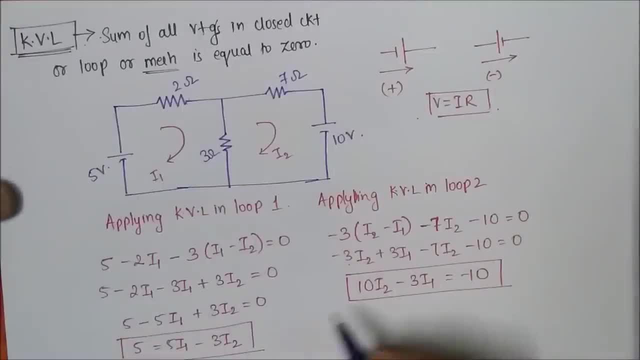 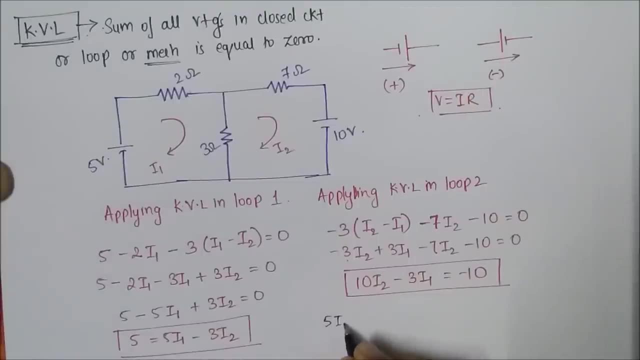 resistance. now I'll be teaching you how to write directly this two equation. if you are in loop 1, add both the resistance. 3 plus 2 is 5, so I'll write: 5 I 1. this registers come under this loop also and it has another. 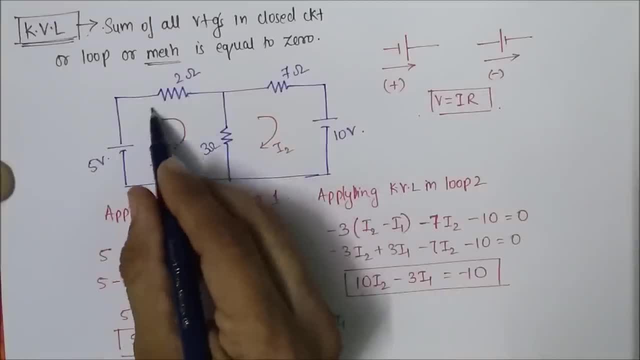 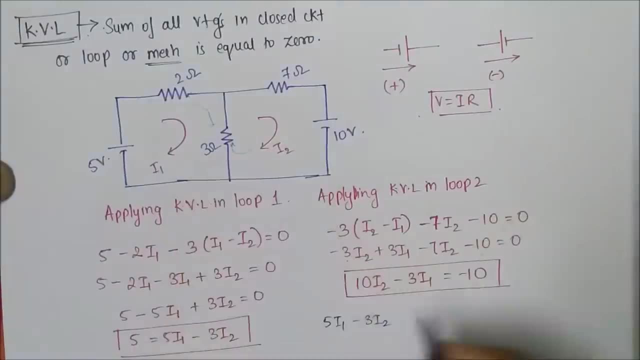 current I 2 and I 1 and I 2. see, you can see I 1 and I 2 are in opposite direction. I'll write minus 3 I 2, because the value of resistance is mine, equal to if I move from negative to positive. 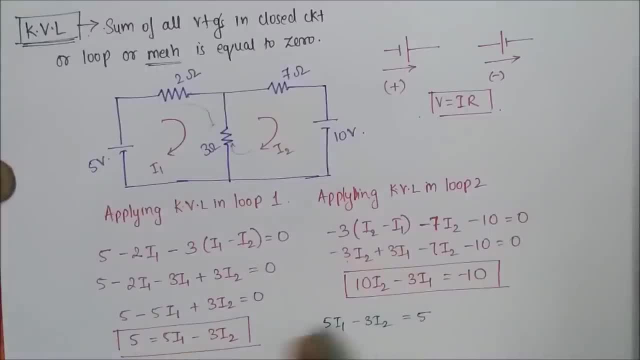 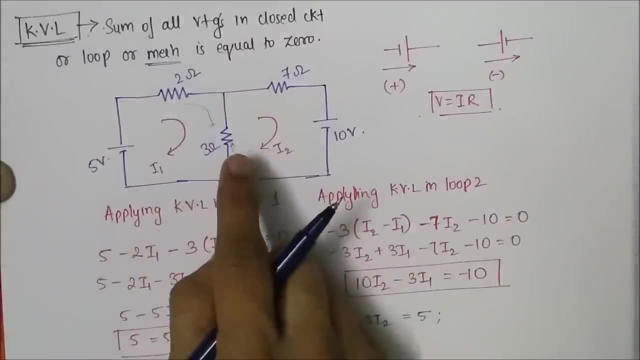 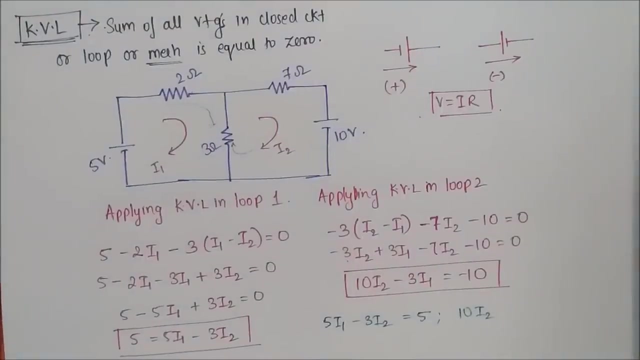 right positive equal to 5. see, we can directly write this equation with the shortcut. similarly, you can attempt this. ok, see, let's I'll show you. we are in second loop. 7 plus 3 is 10. I'll write 10. I to 10. I to the sessions. 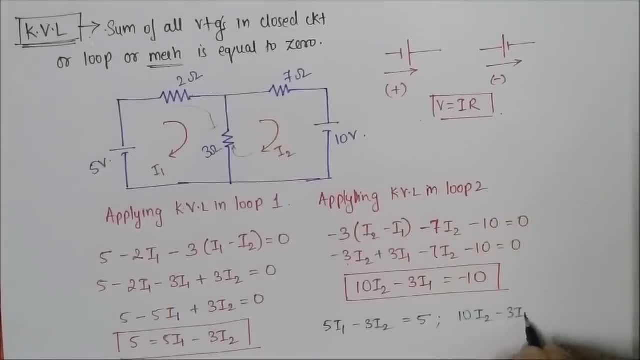 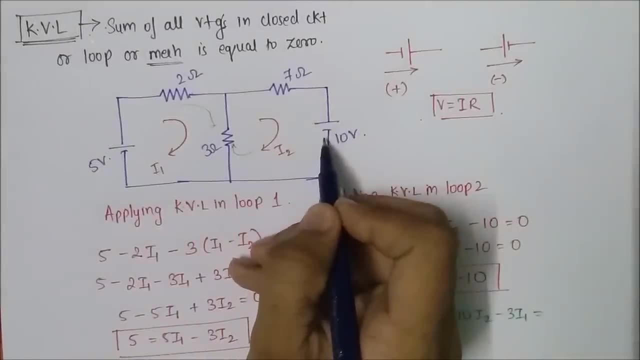 come under this loop also I'll that minus 3i 1 is equal to see in this loop we are moving from positive to negative that's why will write minus 10 then that is � Еще, another minus upgrade to superior temperature so that's why I will write the expression subtract the 2 from 2 and 1 is equal to 5 this is equation we have been doing the equation in second loop 11,1 I'll write 10 i' 2 and 10 i 2 this registers come under this loop also and this number is left. 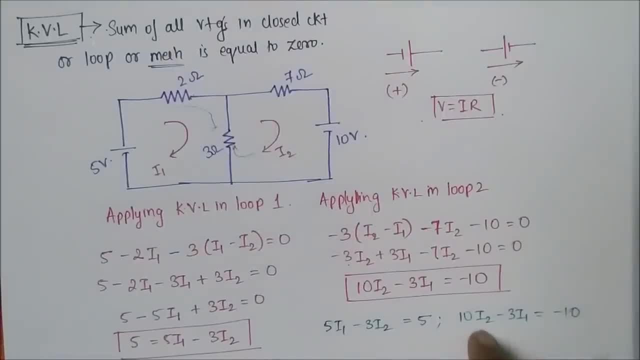 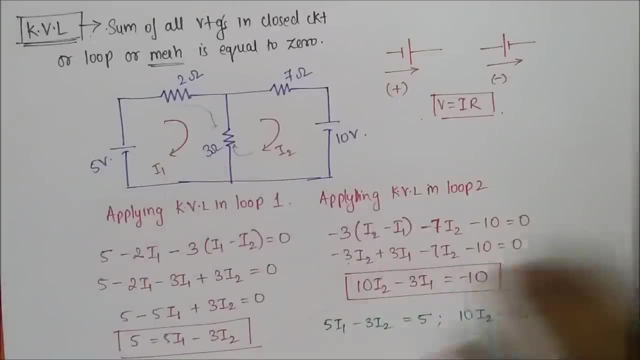 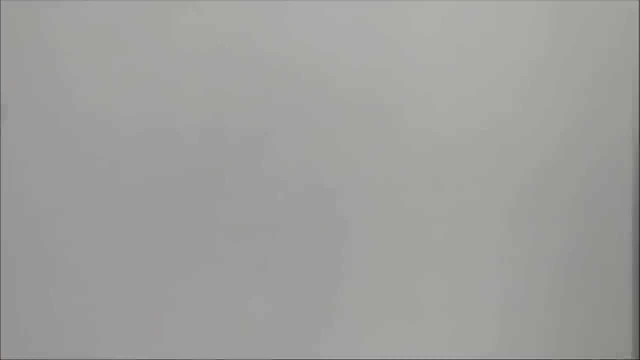 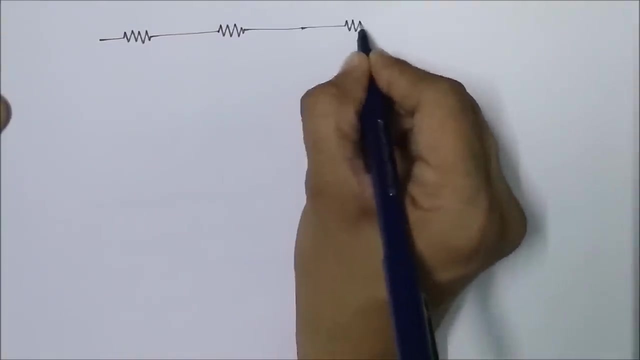 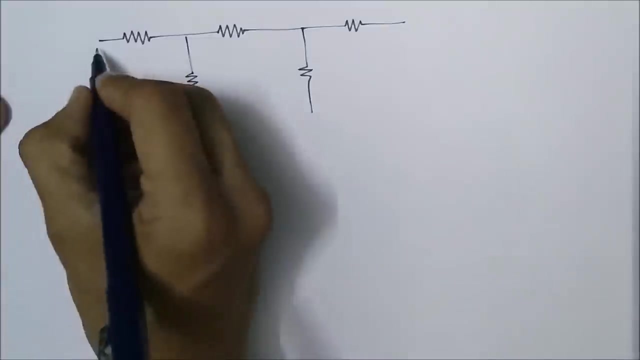 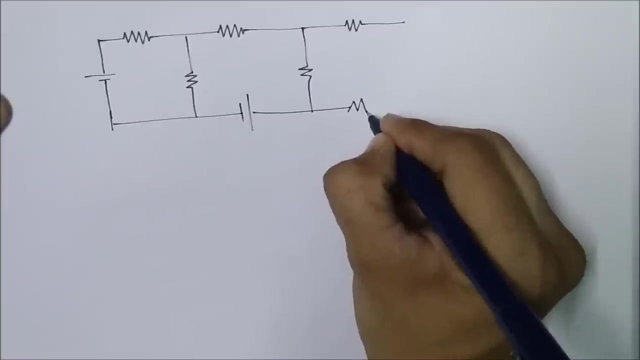 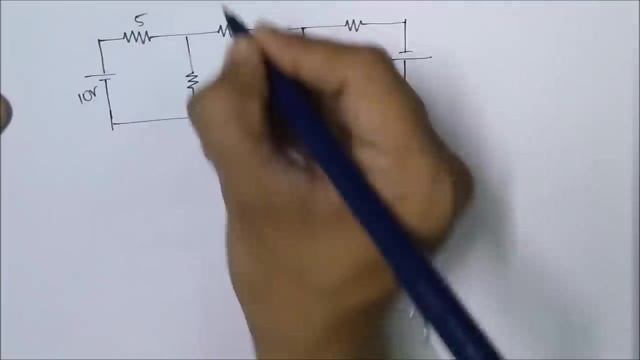 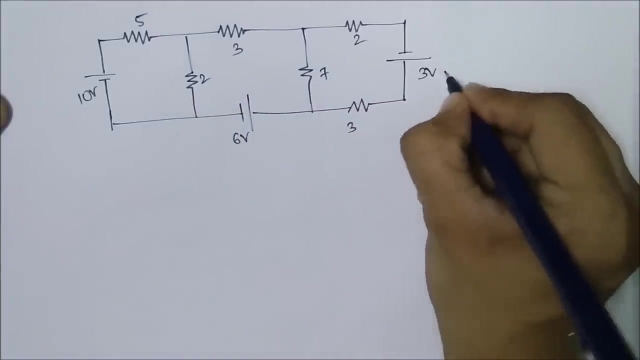 will write minus 10, so you can write directly the equation using any circuits. okay, finally, I'll write. I'll take one big circuit of three loop and I'll try directly writing the equation. okay, so let's take another circuit. take any value of voltage: 10, 5, 2, 3, 7, 2, 3, 6 volt and 3 volt. see now it will be. 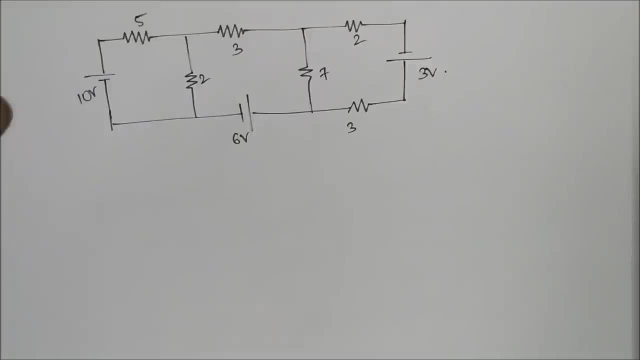 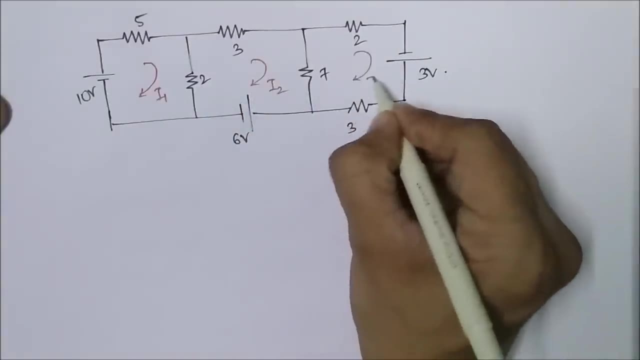 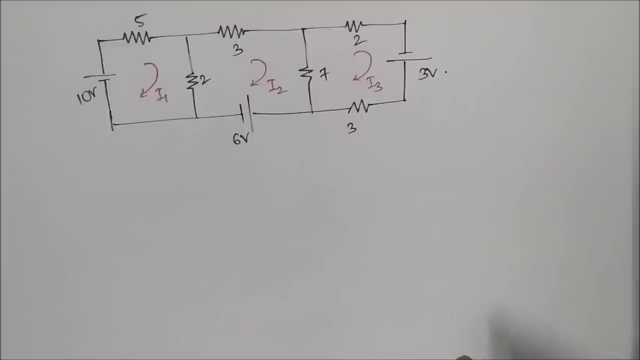 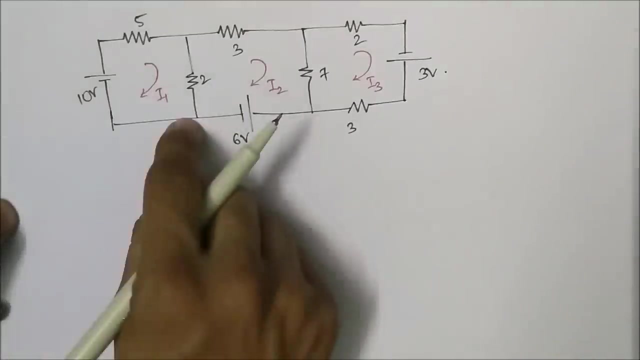 writing directly the equation that we can understand. okay, you, you, this will. I'll take as I 1, I 2, I, 2. make sure I'm making all the equation in the direction of current and the direction is clockwise. okay, you can take any clockwise, so I'll write directly the KVL equation of first loop. okay, so applying. 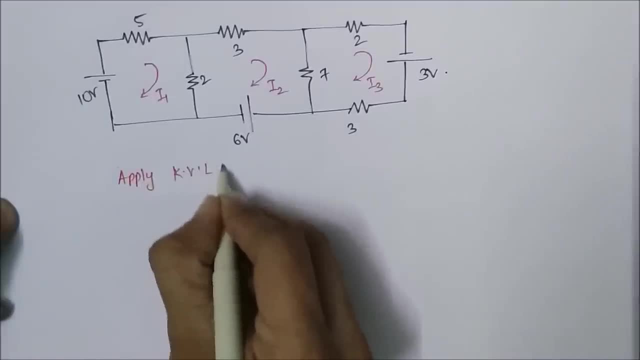 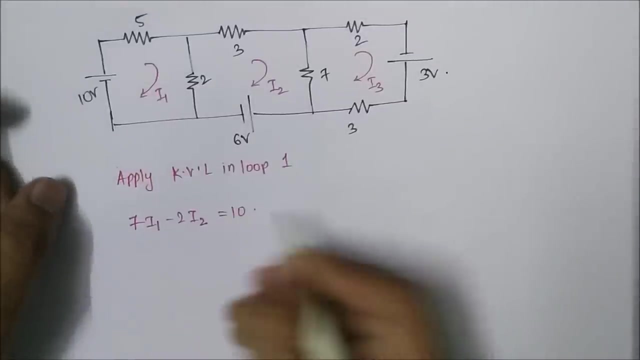 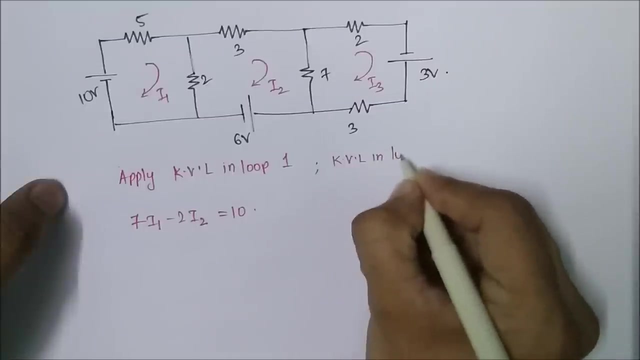 KVL in loop 1. okay, guys, first sequence: 5 plus 2 is 7, I one this existence, Commander, this world. minus 2, I do negative, 2, positive, you are moving. you should write plus 10, or very simple. so can you attempt for 2? KVL in loop 2. come on, guys, for tofu doubt. 2 plus 3 is. 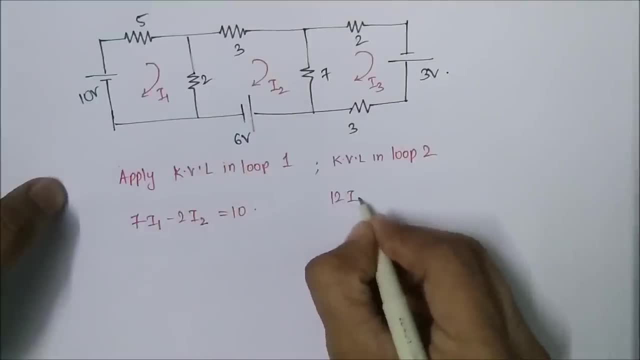 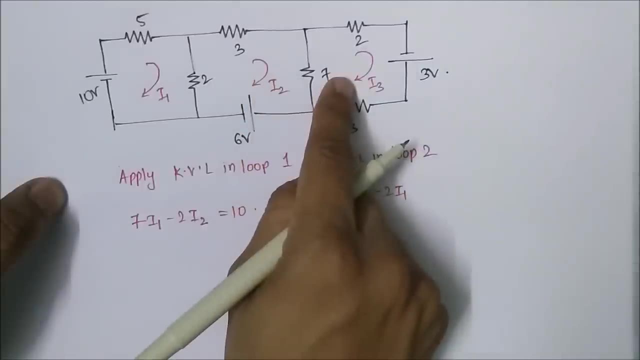 7 plus 3 is 10. 10 plus 2 is 12. sprint to LI to this resistance: come under i1. sell at minus 2: i1. this resistance comes under third loop. very good, minus 7: i3: equal to positive to negative.